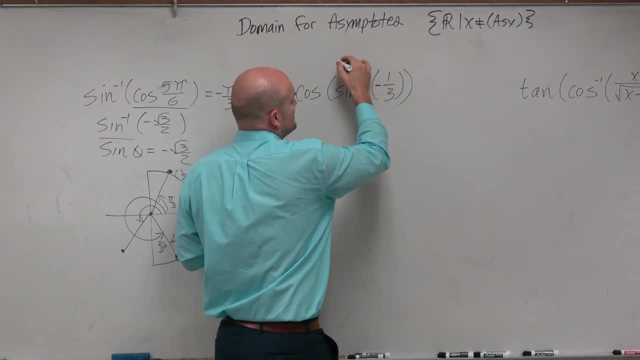 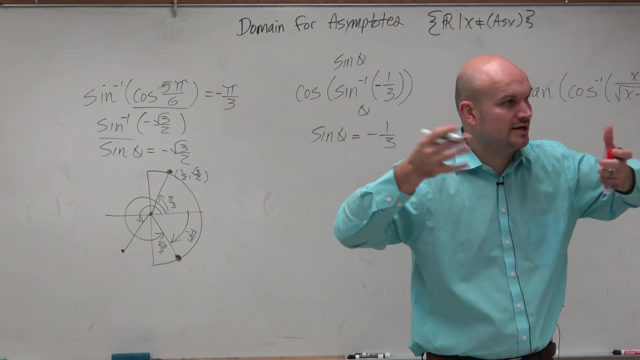 the unit circle Because, again, think about it this way, This is saying the sine of some angle- Actually, I don't remember. The sine of some angle is equal to a negative 1 over 3.. Now again, remember what sine even represents, Like everybody's so focused on the y-coordinate, the x-coordinate, 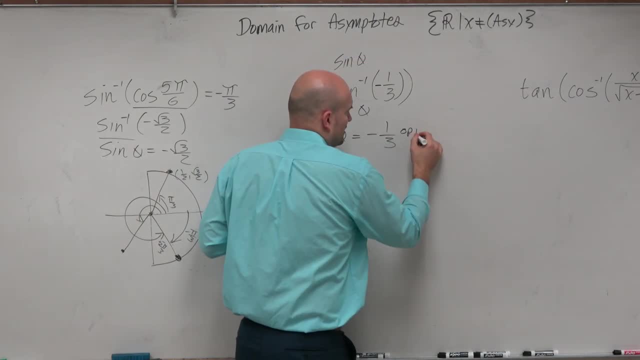 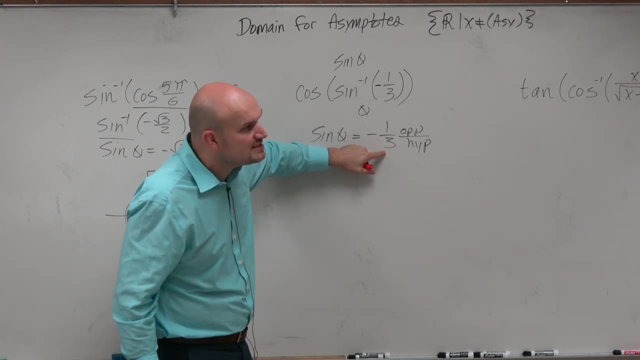 and from unit circle stuff, But don't forget the basics: Opposites over hypotenuse, Right? Obviously, guys, if the hypotenuse is 3, we can see that this is not on the unit circle, Right, Or at least this is not going to be a value on the unit circle. So now that we're 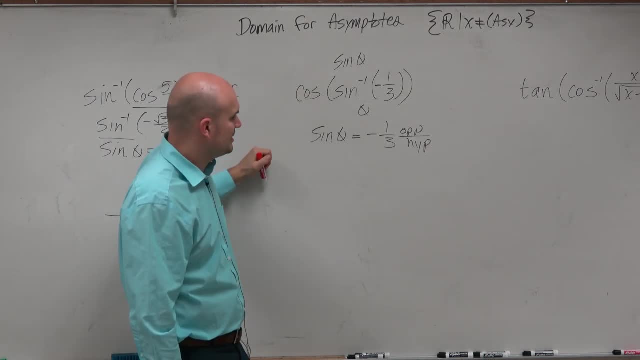 going to be looking at this, or at least for a coordinate point. we're not going to have this y-value, or this isn't going to represent a y-value on the unit circle. So what we want to do now is we can't evaluate for theta unless we had a calculator. But 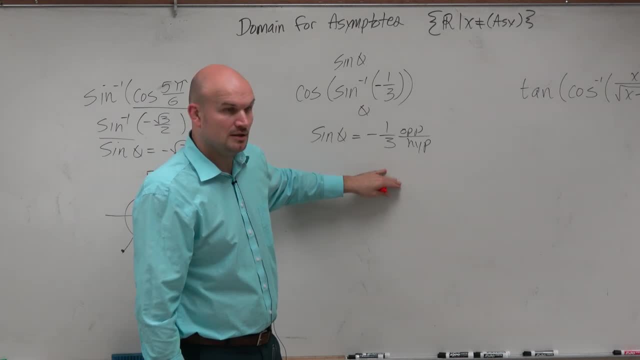 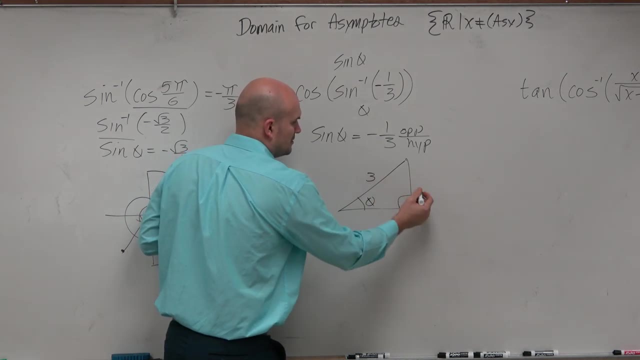 can we draw a triangle that at least represents this relationship Right? So we wouldn't want to do this. Please don't do this Right, Because obviously you're not- not you like. we don't want that to be negative. 1 or don't do that because. 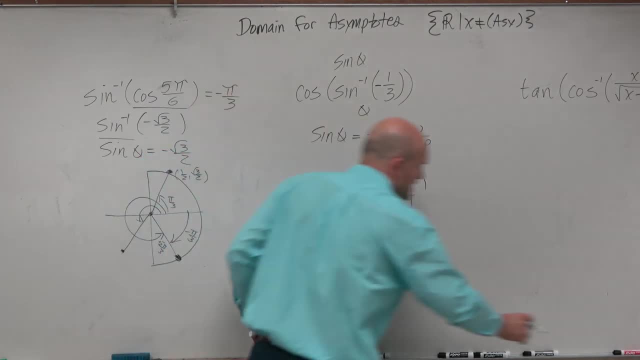 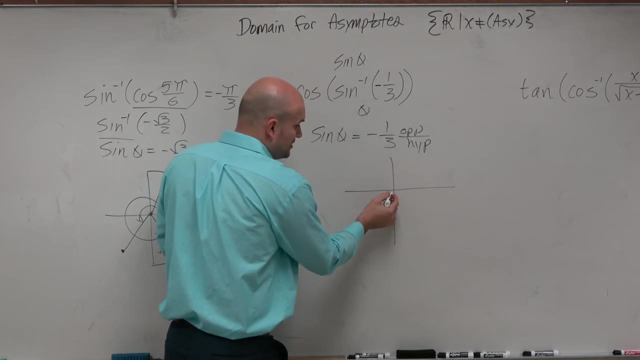 that's a hypotenuse, but we know that sine needs to be negative or the y coordinate needs to be negative, so that means restrictions exist. so there's basically, if you guys remember- this is a good review for your chapter test- there's two triangles that we can create with that central angle: theta negative 1. 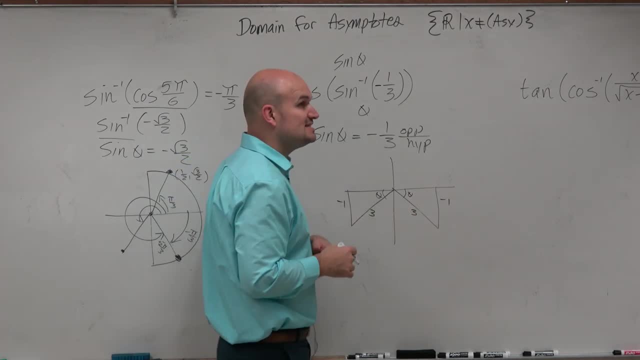 3 and negative 1: 3. now, based on our restrictions of sine, what is the only triangle that's going to work? this one right. so instead of it being a unit circle, it's a circle. instead of being a unit circle, it's a circle where the 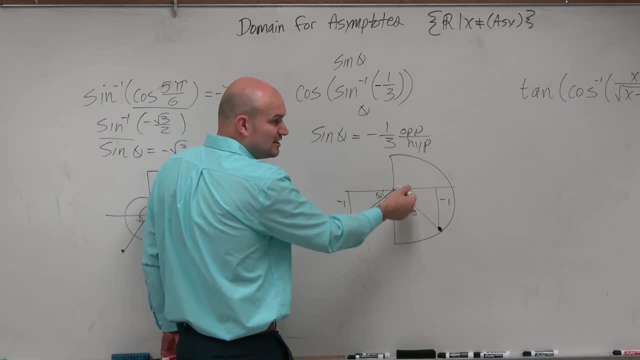 radius is 3, right, so we can't use the unit circle here, but we can still think about this in terms of triangles now. so this is what this creates: this triangle for me. can I, based on this triangle that I created, based on this information, can I now find the cosine of that?